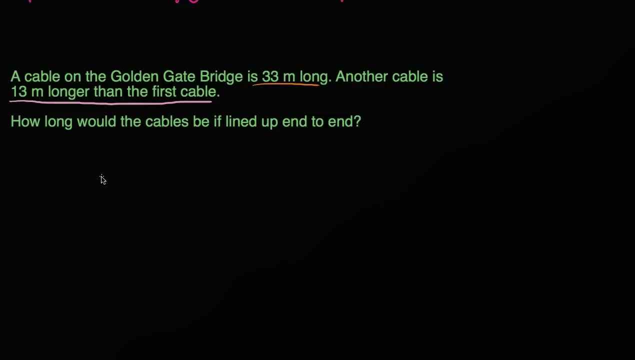 So this first cable is 33 meters. Let me draw it this way. So the first cable is 33 meters long, 33.. Actually, why don't I draw it? why don't I draw it this way? because this is what the cables would actually look like. So this cable is 33, 33 meters long. Another cable is 13 meters longer than the first cable, So this other cable right over here is 13 meters longer. So this cable right here is 13 meters longer. So what's the length of this cable? 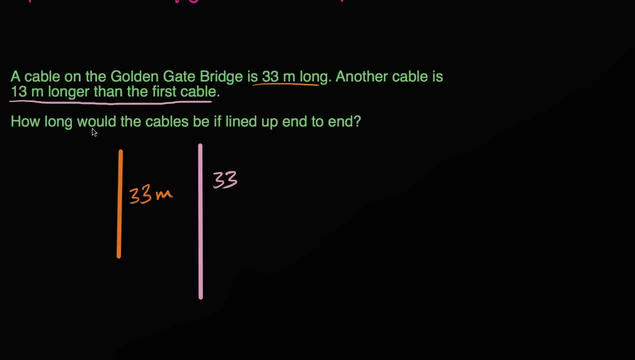 Well, it's going to be the length of the first one: 33, plus 13.. It's 13 meters longer Plus 13,. that gets us three plus three is six. three plus one is four. This one over here is gonna be 46 meters. 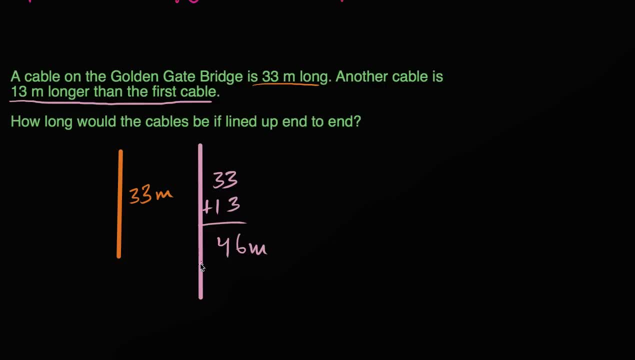 Now they didn't just ask how long is the second cable, which is 46 meters. They're asking how long would the cables be if we lined them up end to end? So if we lined the 33 meter one? so if we lined up the 33 meter one? 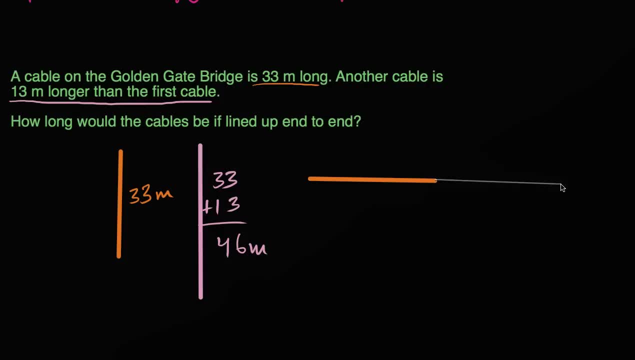 and then, right next to that, we, right next to that- put the 46 meter one. So if we did something like that, well, we know that this one over here is 33 meters and the next one is 46 meters, So we would have to add 33 plus 46. 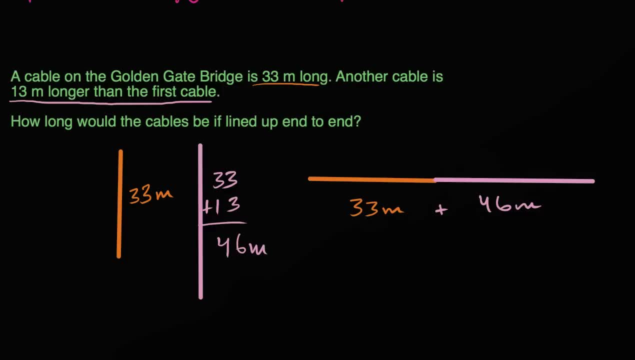 to figure out how long they would be end to end And what is that going to be. So if we say 33 plus 46, plus 46,, three ones plus six ones is nine ones. Three tens plus four tens is 79.. 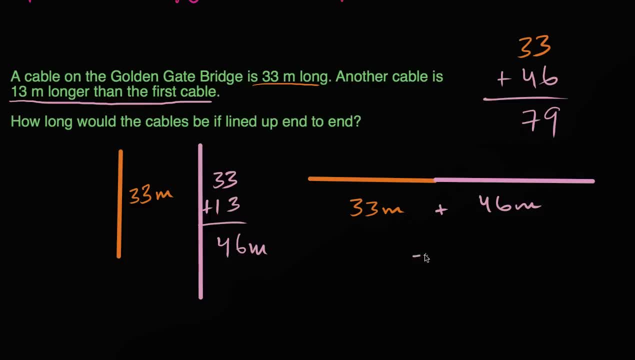 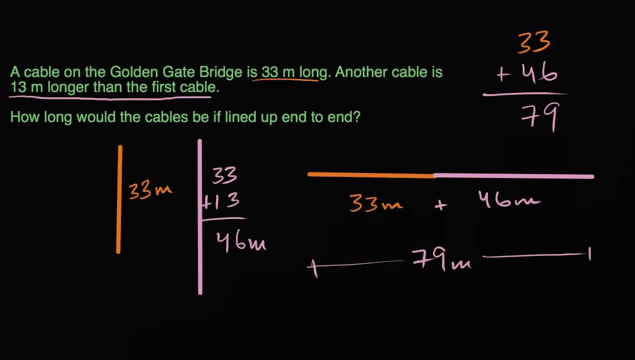 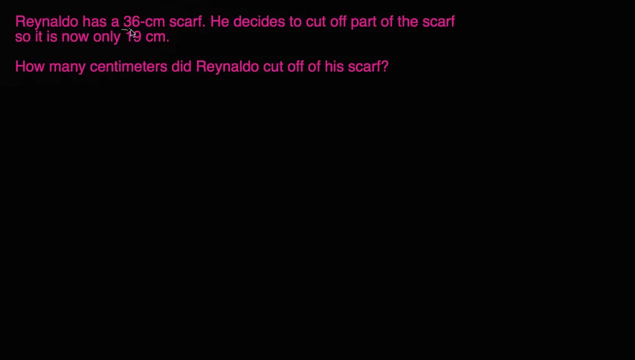 Three tens plus four tens is seven tens, So it's going to be 79 meters if we line them up end to end. Let's do one more. Ronaldo has a 36 centimeter scarf, So he has a 36 centimeter scarf. 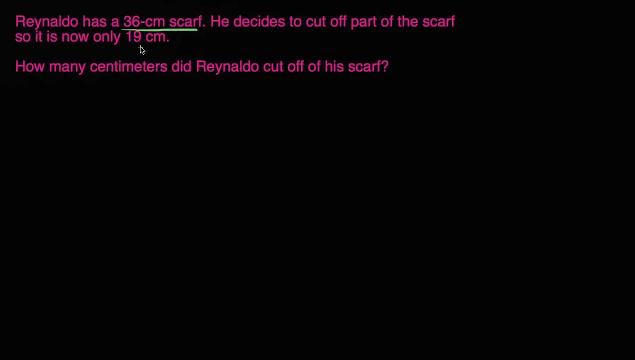 He decides to cut out part of the scarf, so it is now only 19 centimeters. How many centimeters did Ronaldo cut off of his scarf? So let's draw his scarf. So it was a 36 centimeter scarf, so it might have looked something like this: 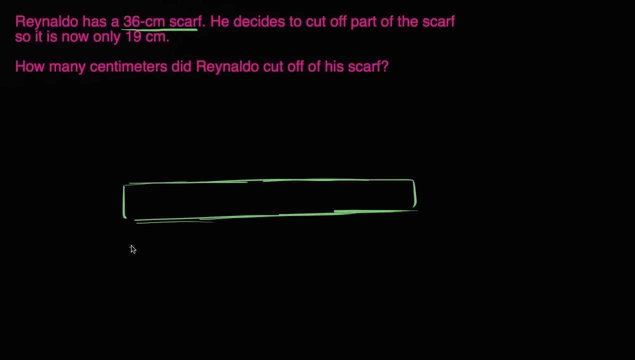 So this was his scarf before, if I stretch it all out, And it is 36 centimeters. 36 centimeters long, But he cuts part of his scarf, so it's only 19 centimeters long. So now it is only 19 centimeters.